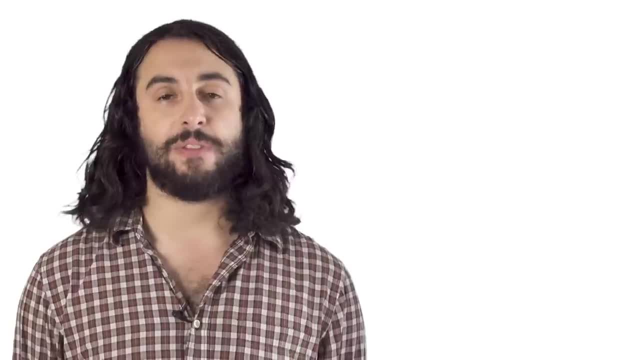 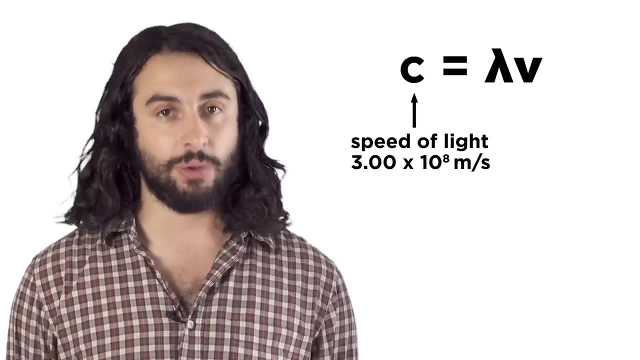 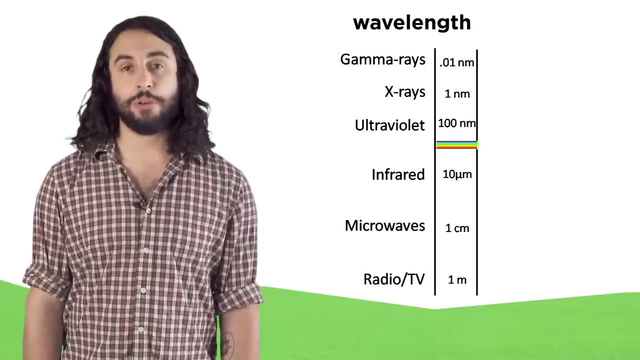 higher frequency. these variables are related by the following equation, in which C is the speed of light, about 300 million meters per second, the speed limit of the universe. the electromagnetic spectrum shows light of all the different wavelengths, from gamma rays to radio waves, including this tiny 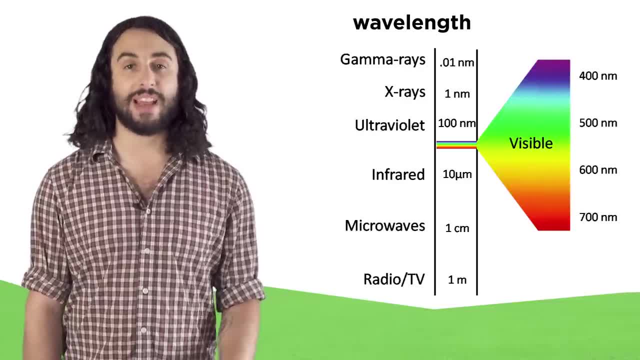 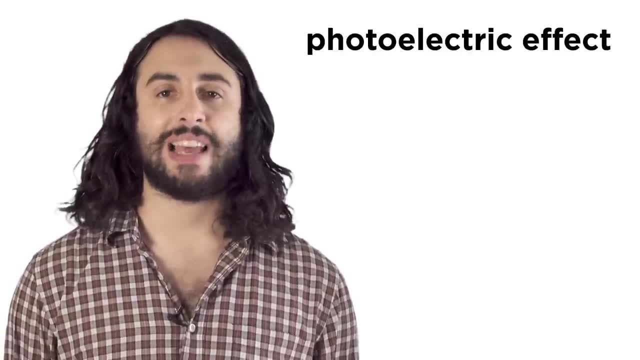 sliver in the middle which is visible light, the light we can detect with our eyeballs. the wave theory of light was very useful for a time, but it could not explain the photoelectric effect. this was the observation that if a certain metal plate is irradiated with light, an 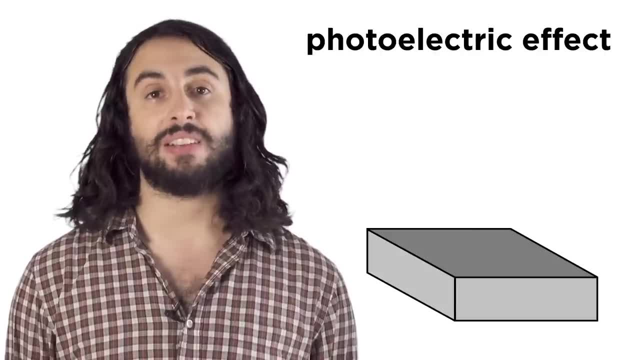 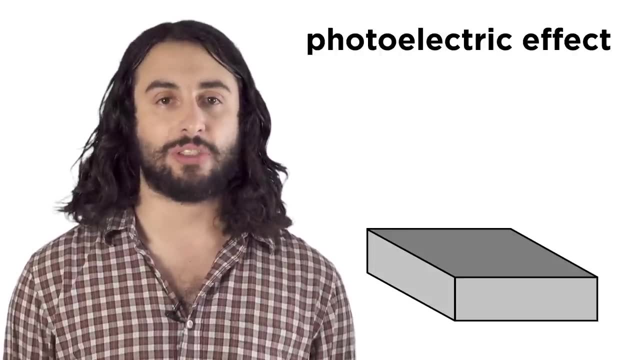 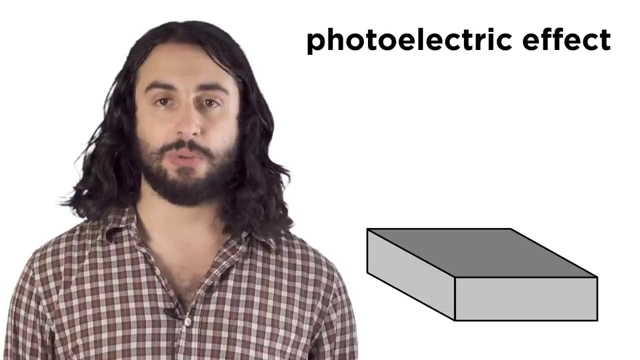 electron is ejected, which can be detected when it interacts with a positively charged wire or plate sensor. the incongruity was that the ability of the light to eject an electron depends only on its frequency and not its intensity. so if the beam was below a certain frequency, even a very intense beam with 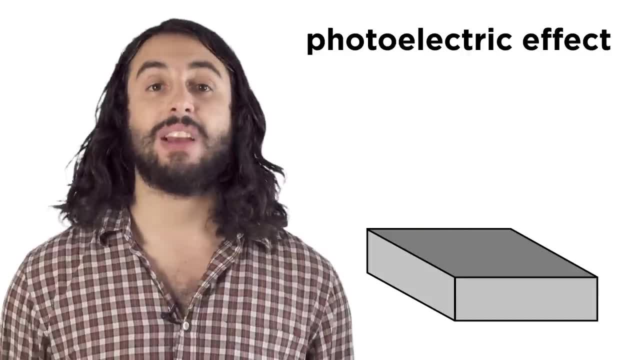 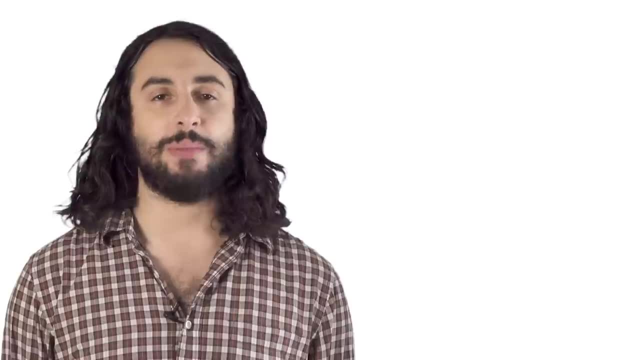 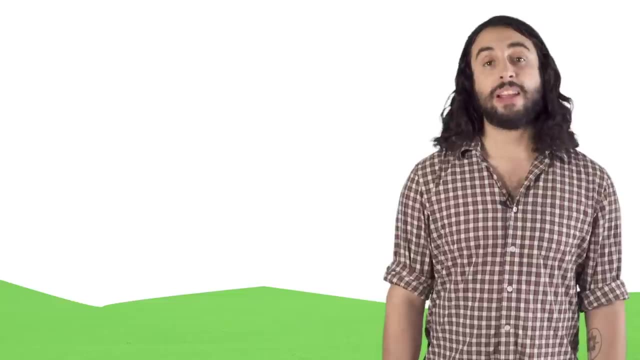 a lot of light could not eject an electron, whereas above a certain frequency the faintest beam possible could do it. this seemed strange, and a famous fellow named Albert Einstein solved the problem by extending a concept developed by Max Planck just five years prior. Planck proposed that 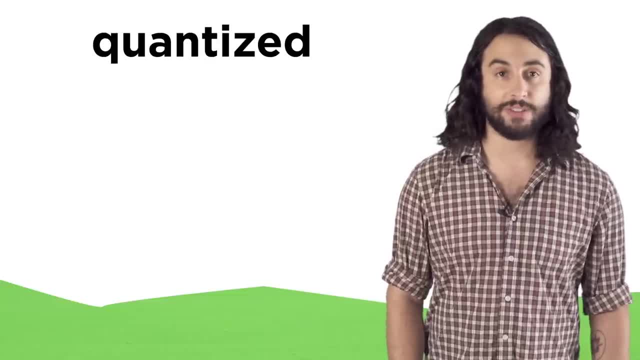 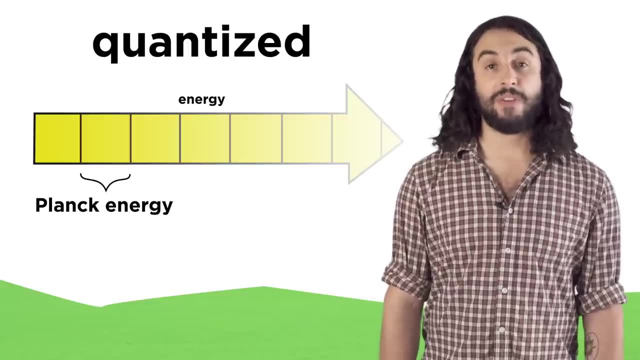 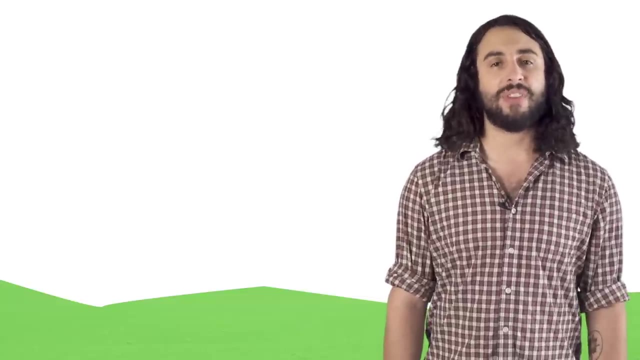 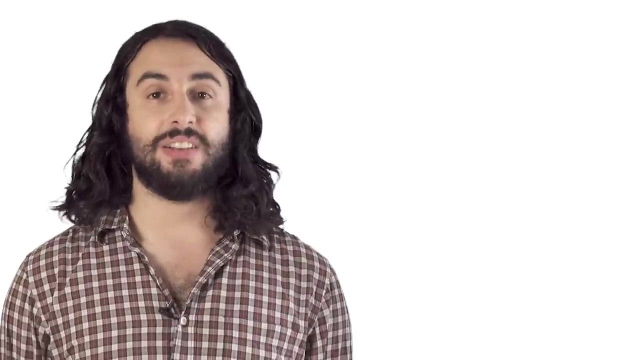 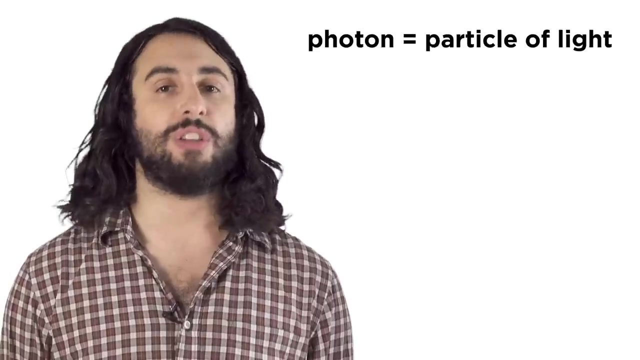 energy is not continuous, but rather is quantized. that is, all energies are multiples of the small number of light. Einstein explained that light must also be made of quanta, which he called photons. these are particles of light. this explained the photoelectric effect. 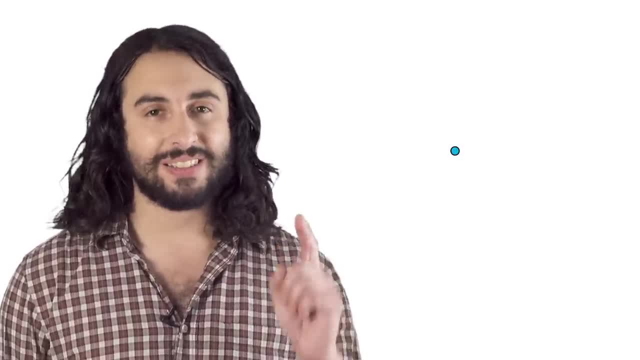 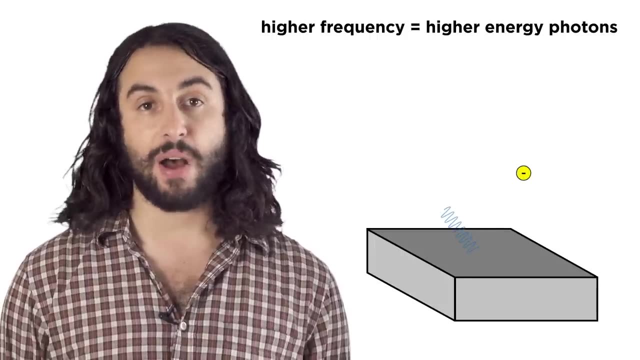 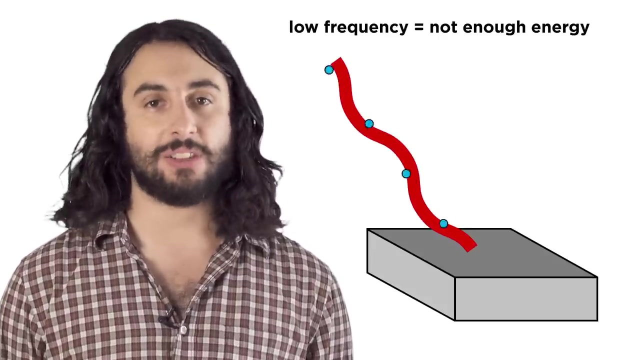 because an electron is ejected when struck by a singular photon with sufficient energy. it only takes one photon. so even the faintest beam above a certain frequency will be able to do it. but if none of them are of that minimum energy, no matter how many photons strike the sample, an electron will not be. 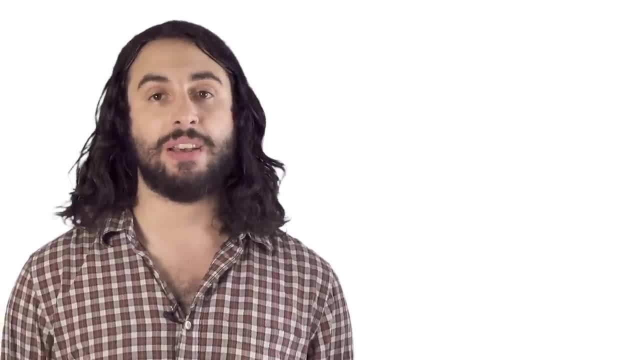 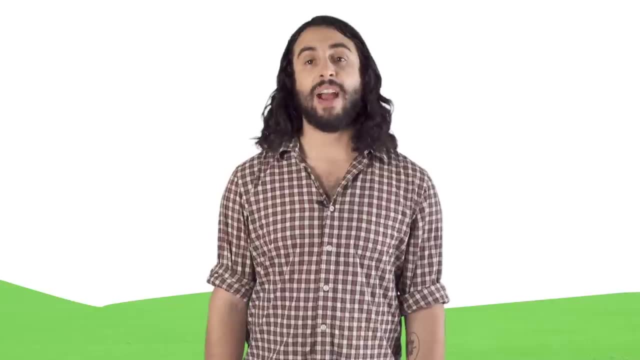 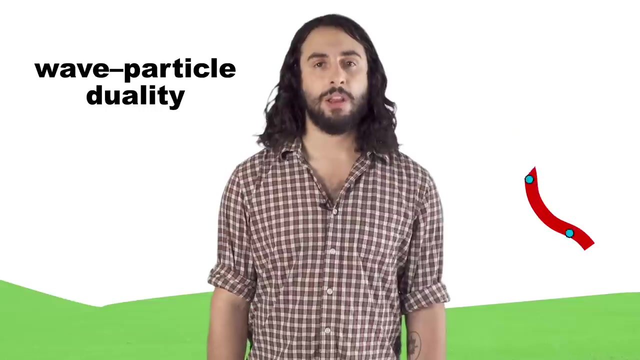 ejected. it was found that the energy of a photon can be given by the following equation: according to the frequency of the photon and Planck's constant. we now have to accept that light obeys wave-particle duality, meaning it is both a particle and a wave at the same time. confused you should be. this is the.